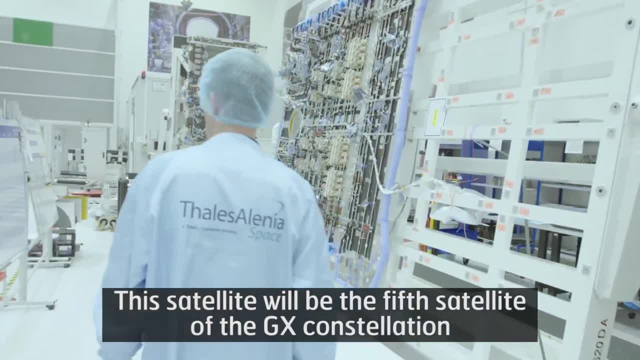 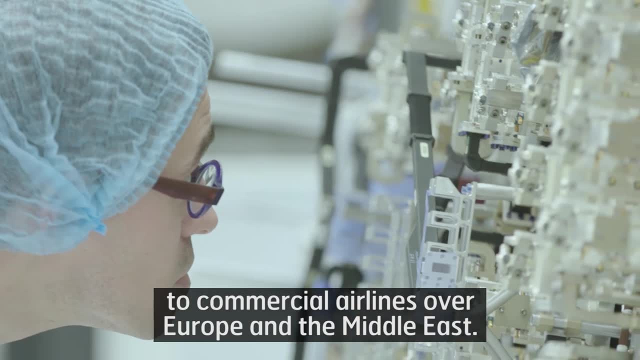 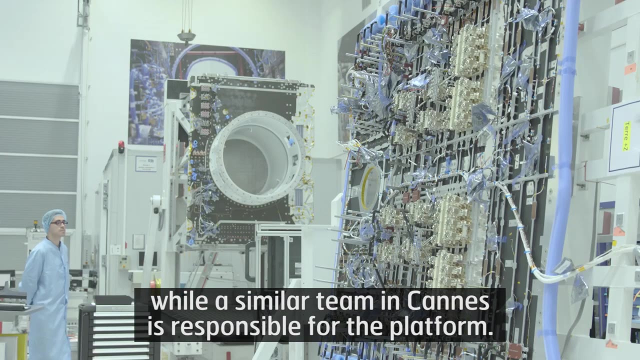 This satellite will be the fifth satellite of the GX constellation, and its main function will be to deliver Wi-Fi to commercial airlines over Europe and the Middle East. The work we do here is mostly related to the payload of this satellite, while a similar team in Cannes is responsible for 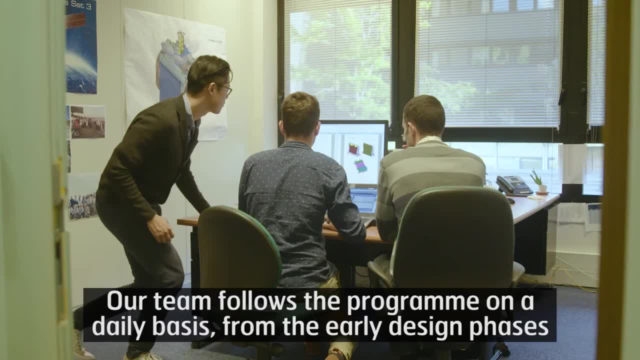 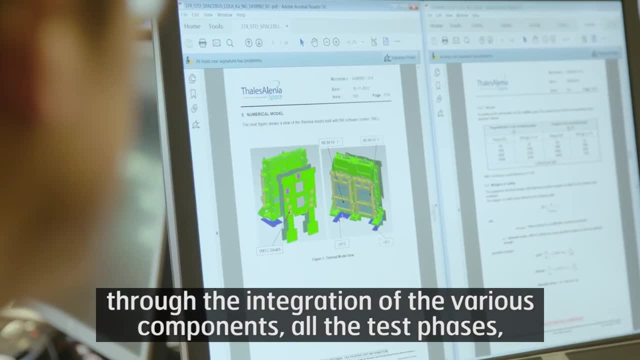 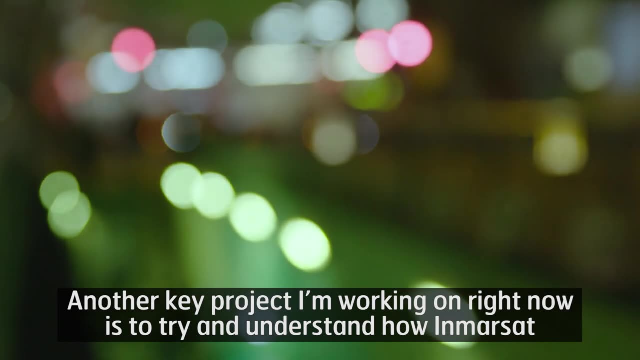 the platform. Our team follows the program on a daily basis, from the early design phases through the integration of the various components, all the test phases, launch and in-orbit testing. It's a fascinating job. Another key project I'm working on right now is to try and understand. 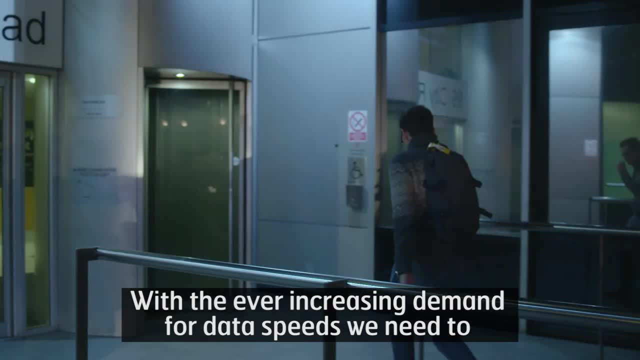 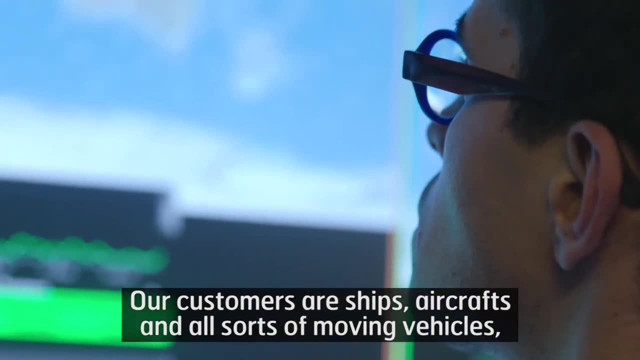 where and when new capacity will be needed. With the ever-increasing demand for data speeds, we need to anticipate capacity deployment far in advance. Our customers are ships, aircrafts and all sorts of moving vehicles, so we need to know where and when new capacity will. 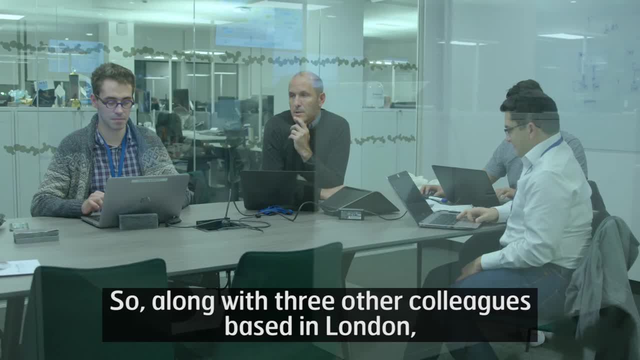 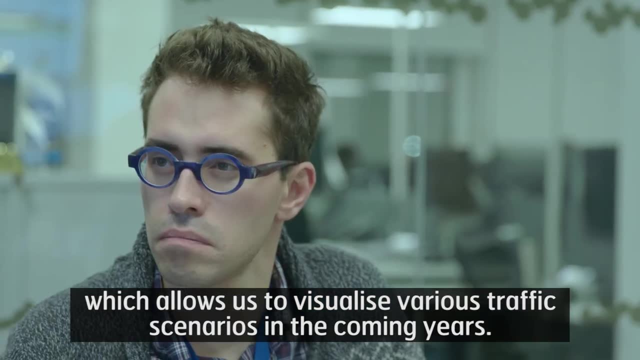 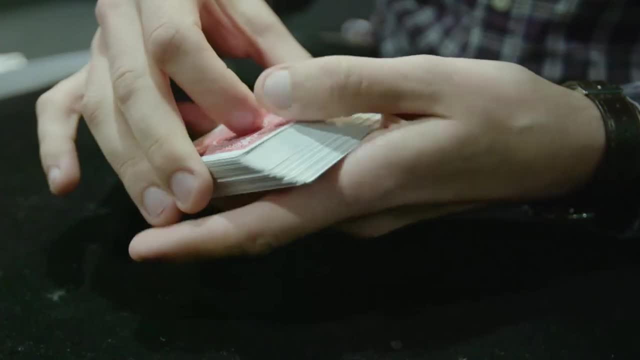 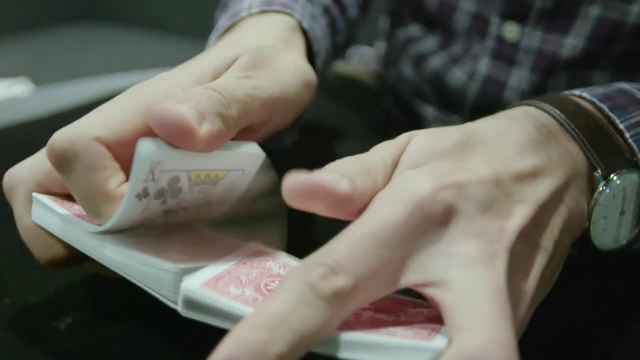 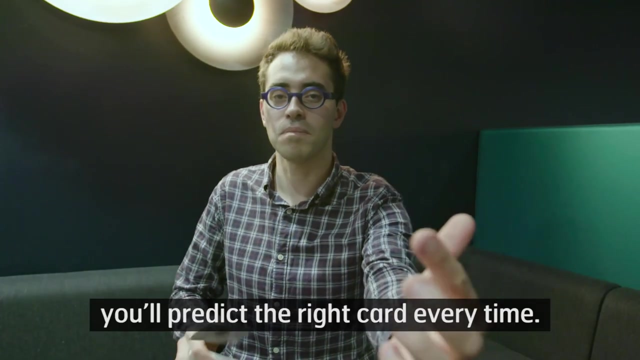 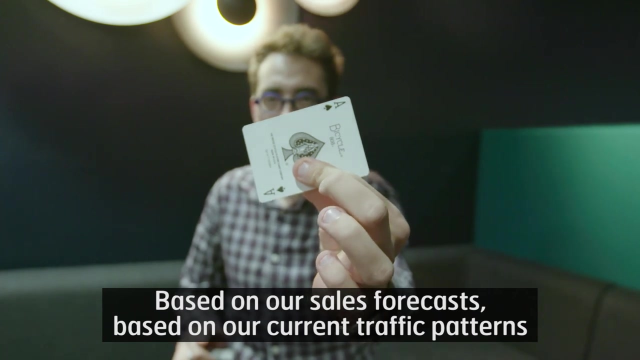 I like to write, I like to write, I like to write And in some ways this project reminds me of that, But of course it's not magic. If you understand the method and the moves, you'll predict the right card every time, Based on our sales forecasts, based on current traffic. 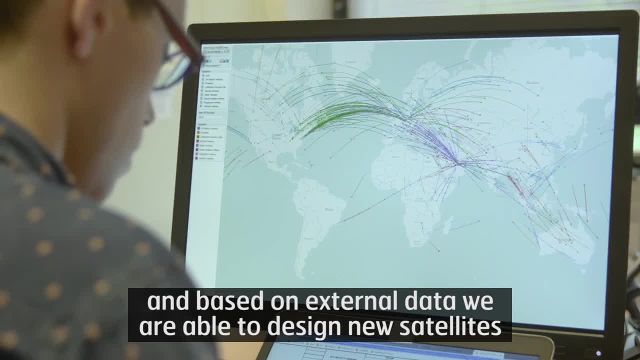 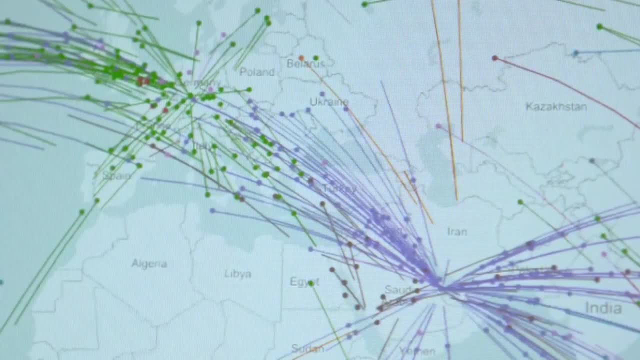 patterns and based on external data, we're able to design new satellites and new coverages to augment our current capacity where and when it will be needed. So the awesomeness of my job lies in being able to follow the whole story from the moment. 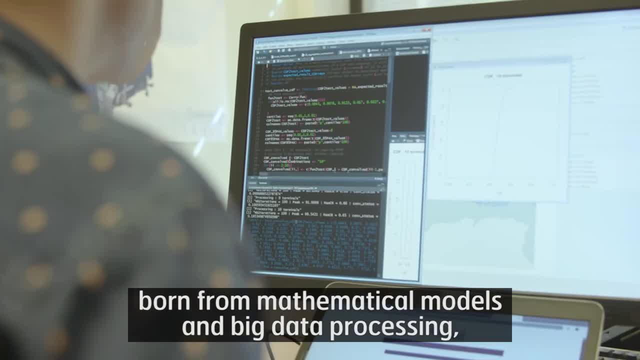 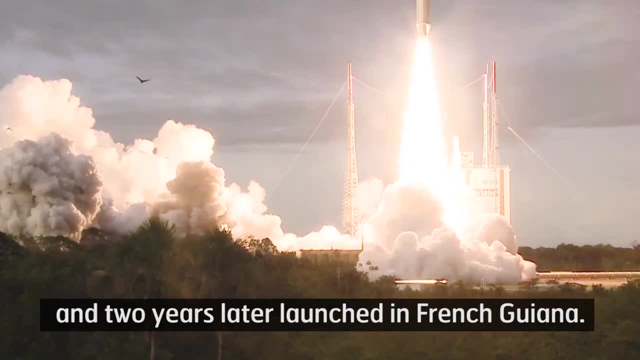 when the satellite is barely a preliminary concept, born from mathematical models and big data processing, to the moment when it's actually being built here in Toulouse and, two years later, launched in French Guiana. For me, no, two days are the same, and for that reason, I love my job.